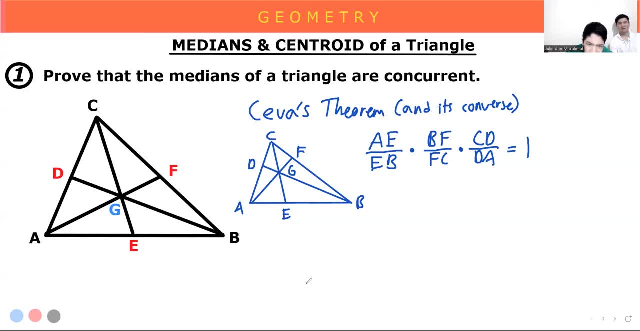 us that the chevians are all concurrent. So a median is a chevian, but the opposite side is bisected by that chevian Meaning. the opposite side will have two equivalents. It will be divided into two equivalents, So it marks Okay. So 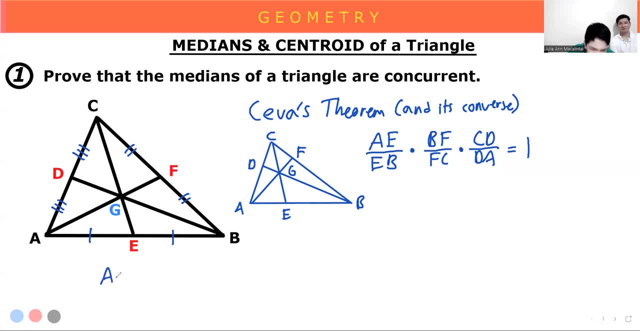 If we can prove that Ae over Eb is times Fb over- Oh wait, Bf, to make it better- Fc times Cb over De is equal to 1. Then we can prove that the medians are concurrent, Since Ae is. 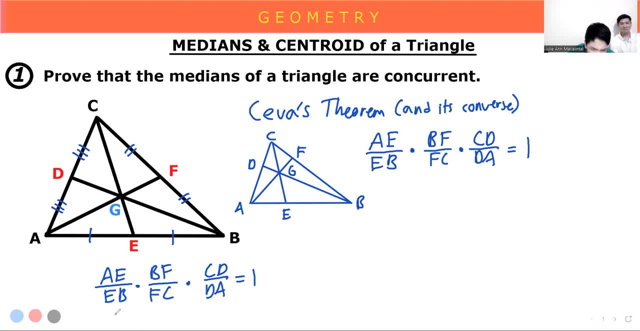 in the figure found to be equal to EB, then this will equal 1 and BF is also tick mark to F3. 1. yes, AA over EB. so if they are the same, their quotient is 1. BF over FC is also 1 because they are. 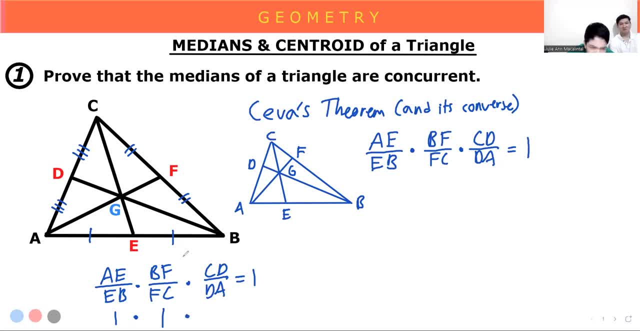 congruent. similarly, CD is congruent to BA, so therefore its quotient must be 1, and 1 times 1 times 1 is obviously equal to 1. so therefore all three medians of a triangle are congruent. so and then, what do you call? 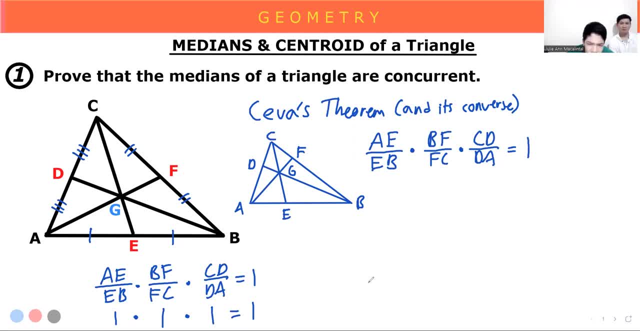 the point of congruence of all three, point of congruence of all three medians of the triangle is called centroid. centroid, yes, if you make, yes, if you make a sheet of paper and then a triangular piece of paper and then label it centroid if you put it. 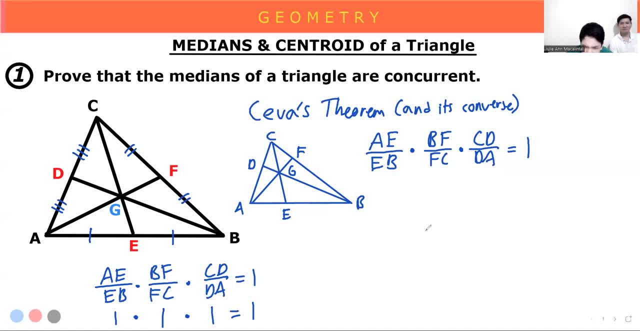 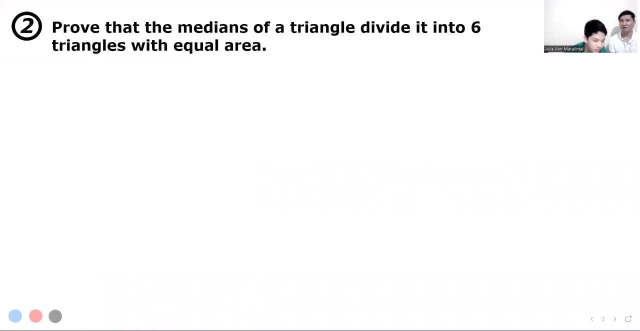 on a pin. it will balance because the centroid is the center of gravity. yeah, okay, let's proceed to number two, but we will be using: are you going to use the same figure? yes, I will be using the same figure, okay, so so quick sketch P: oh I. 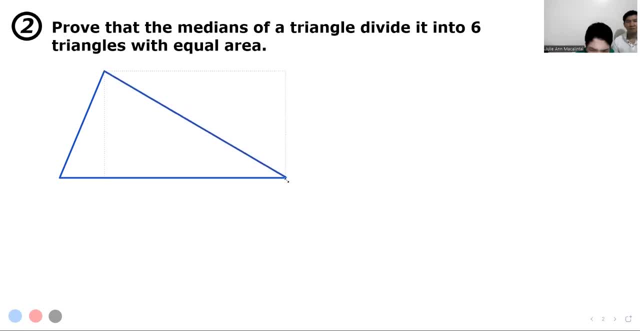 don't know where is my sketch. Yeah, otherwise questions. E There, it looks good. So number two proved that the medias of a triangle divide the triangle into six triangles with equal area. So even just with eyeballing you can already know that they are approximately concurrent. 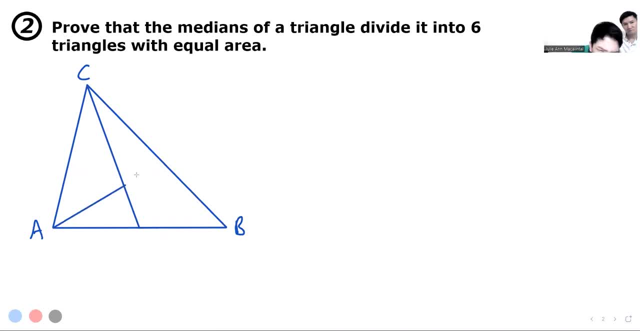 Here I'm only eyeballing what seems to be the midpoint. This seems to be the midpoint, Without even looking at the others. that seems to be the midpoint, And they are. it just seems to be the midpoint, but they are already obviously concurrent. 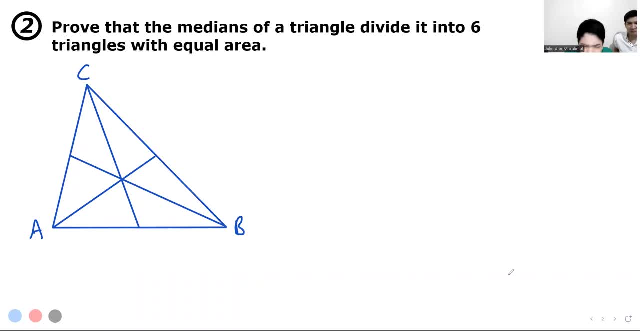 The midpoints, Yes, wait, You will always know when I was using the word Ah, the E, Yes, which one. This is what: The centroid, The centroid. Okay, So I will prove one case first. So maybe we will prove it with the already upright. 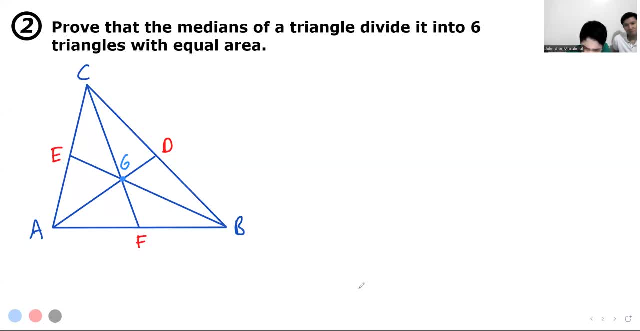 Well, while it's already upright so we don't have to flip it. So I will highlight the triangle A, B and C In the congruent length. Yes, Oops, Yes, Yeah, Almost perfect, Okay, Sola V. 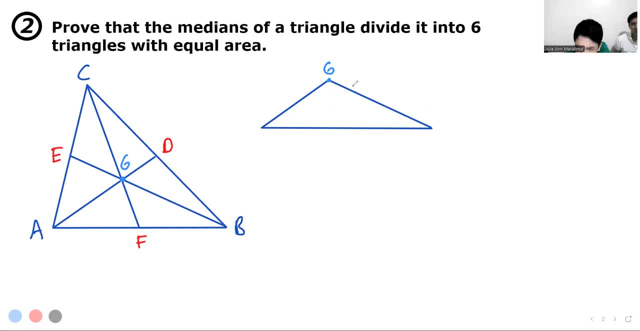 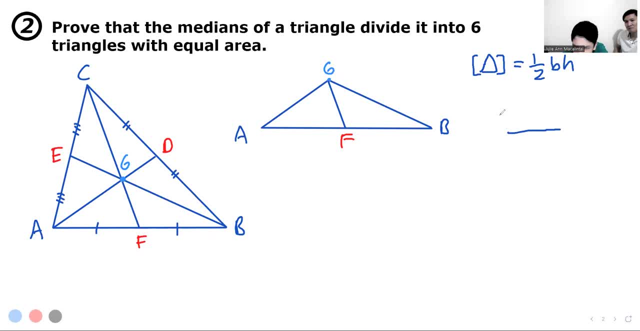 So let's say there are two triangles with the same base and same height. So this is the following: Okay, If they have the same height and the same base, then their areas are equal. This also applies to The base. 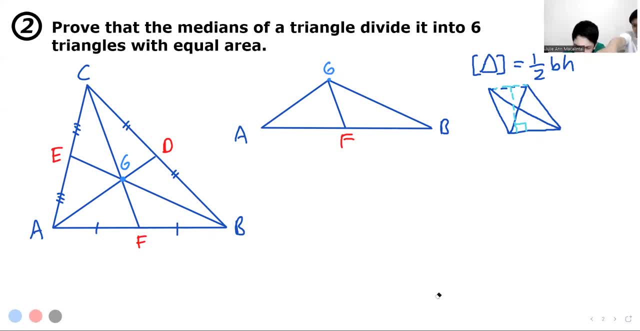 Ah, yes, The base With the bracket. So that's the base. This is the height. So yes, So they will have equal area. If two triangles start from the same height- I say vertex- then obviously their height is the same. 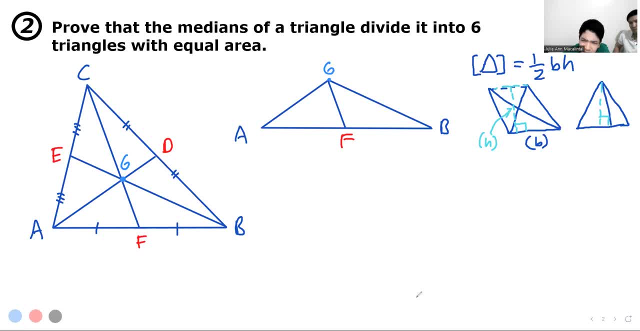 So here two triangles: A F, G and F G B, with A F G A, F G A, F G, And oh, it looks blue, It looks pretty blue there. 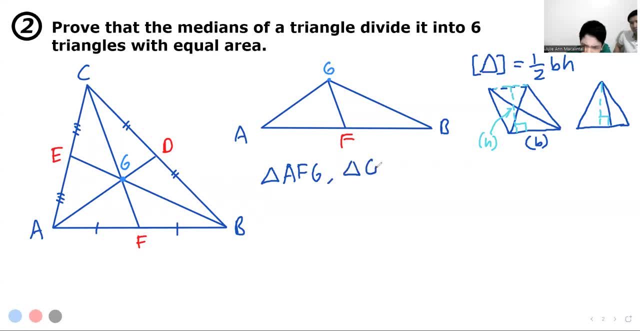 And F, G, B- Okay, Yes, B. They have congruent bases. It doesn't have to be actually the same base, as long as the base is congruent And they have the same height. Their height is the leg. 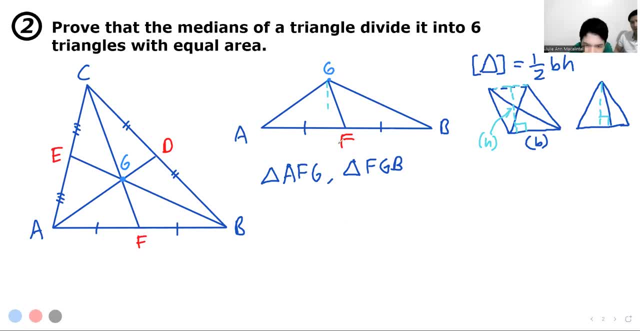 Yes, Yes, Their height is also the same. They have equal heights, Same height And the piece of nature They have the same height. I mean they have the same altitude And equal basis, Equal basis. So therefore, the area of A- F- G is equal to the area of F G- B. 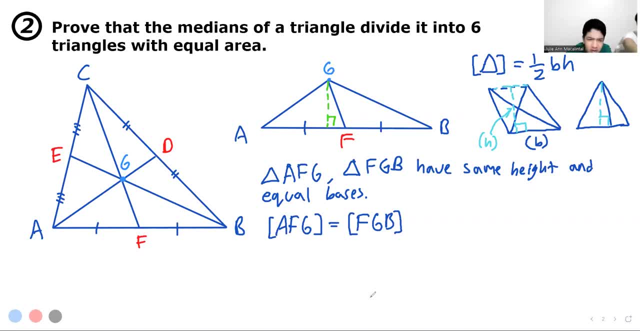 Similarly, I will again highlight: Yes, Yes, Yes, Yes, Yes. This triangle, This triangle, That's the same area, This triangle, Yes, So, similarly, Similarly- Oops, it's still not locked. Similarly, similarly, similar. 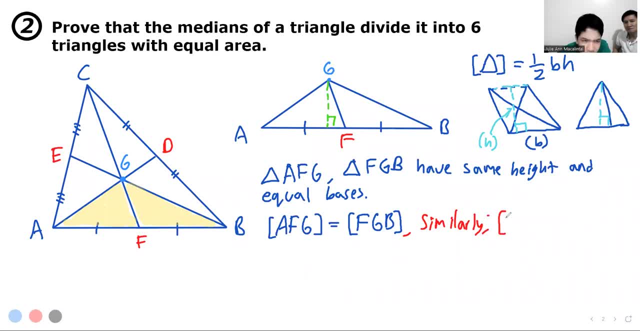 Similarly, the triangles are CGD and GDB. G-A-A, right, C-G-D is equal to G-B-B. It's just flipping. Yes, So something like this: C-B-B-B-B-B-B. yeah, That's a small triangle and this small triangle is equal to G-A-B-B-B-B-B-B-B-B-B-B-B-B-B-B-B-B-B-B-B-B-B-B-B-B-B-B-B-B-B-B-B-B. 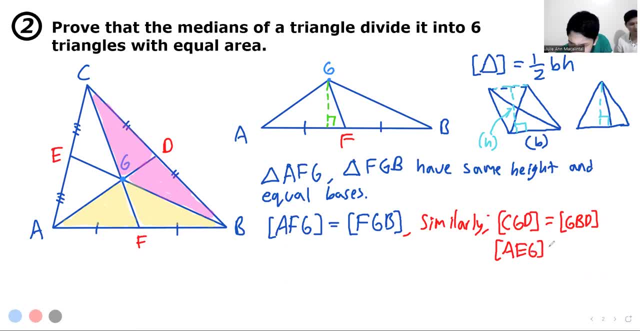 The triangle is G-B-B-B-B-B-B-B-B-B-B-B-B. Probably Now you can understand that The triangle is G-B-B-B-B-B-B-B-B-B-B-B-B-B-B-B-B-B-B-B-B-B-B-B-B-B-B. 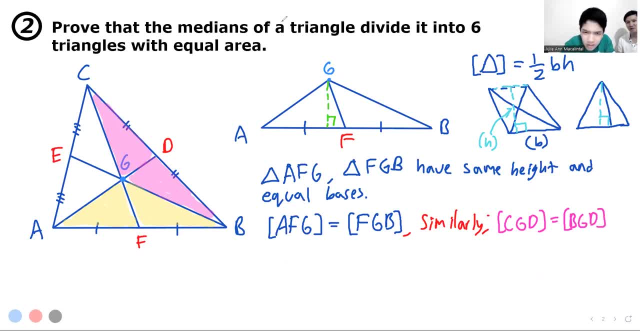 Certainly it's just flipping Same thing. but that is only 2, 3. Great, So it's already 2.. I'm sorry, 15. 13. Yes, so I will scale it down a bit because they are in a circle. 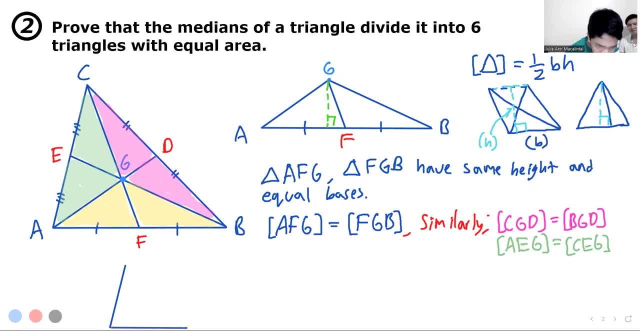 I just zoomed 8 params, Okay, so that was very perfect. Luckily I hope it did come out, And then I'll just move this up Here: C, D, F, B, So again same height, same base. No, not same height. congruent basis. 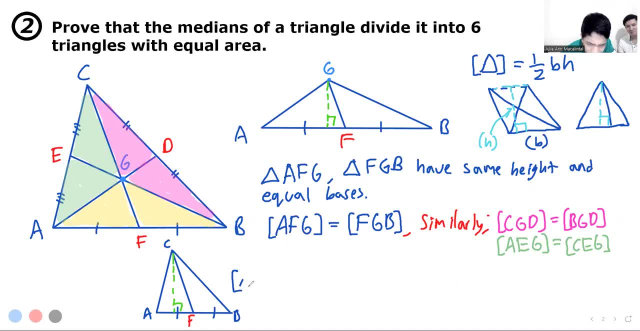 Therefore, E, C, F, Area of ACF is equal to area of BCF. Similarly, I'll just write it in red. There's no error. ACF is equal to No, not ACF. I just wrote it again. 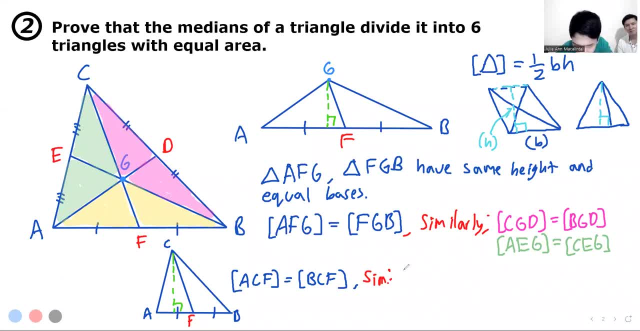 Um, AEB is. Area of AEB is equal to area of CEB And Uh, Area of Yes And for the For BC. When BC was the base, AEB was Yes, Yes. So because of this, 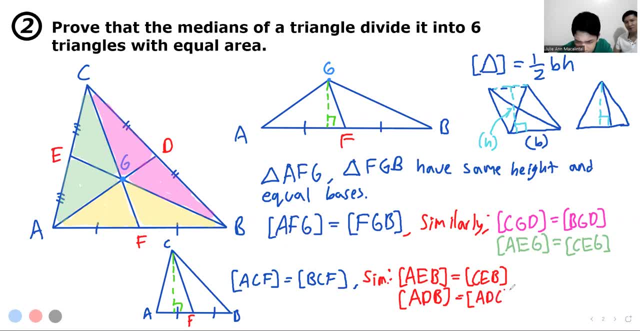 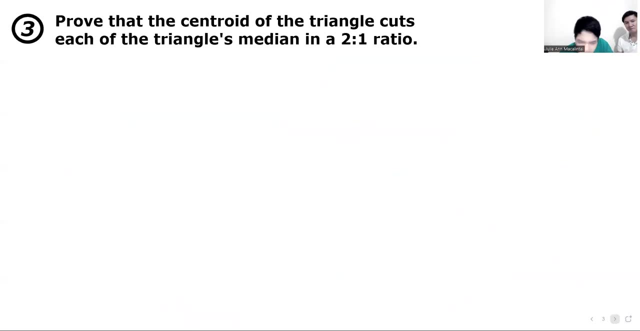 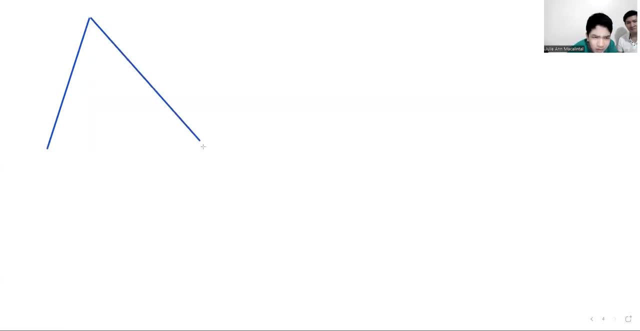 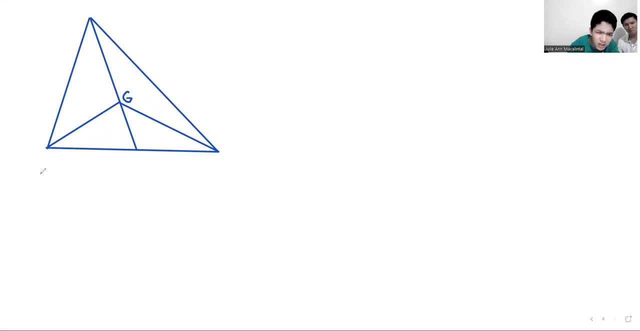 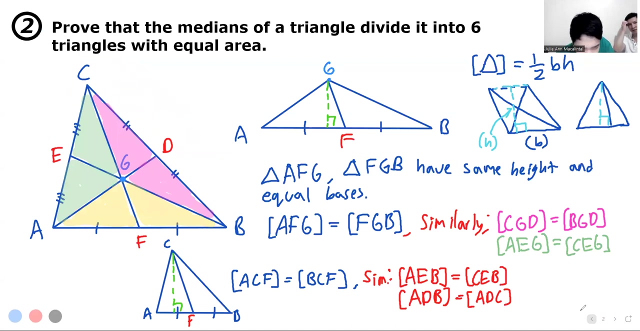 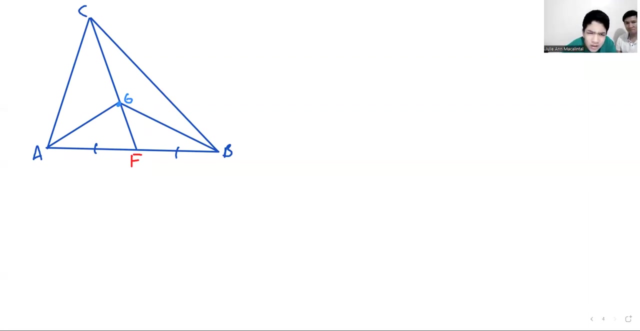 exactly what I was hoping for. G. when did I write it again? G, centroid F, this is ABC. yes, so that yellow area, which is AFG, oops, equal X. okay, let's purple, pink area, pusha area, let's what's that? CGD, BGD, equal Y. 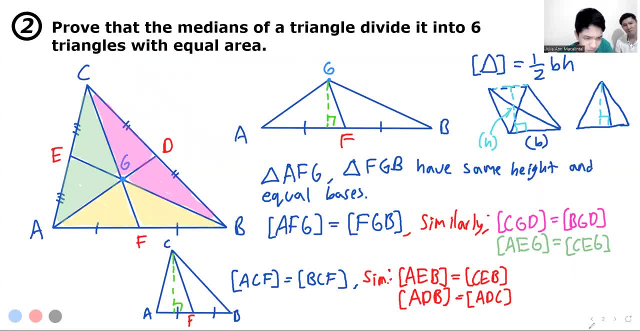 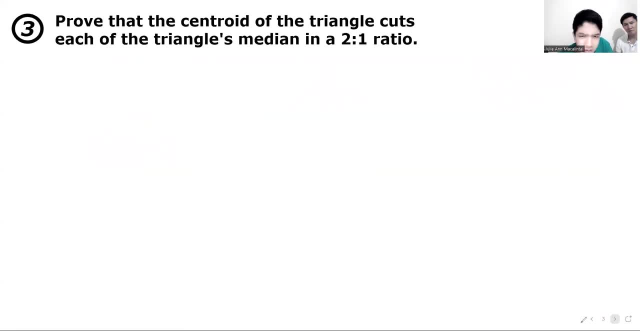 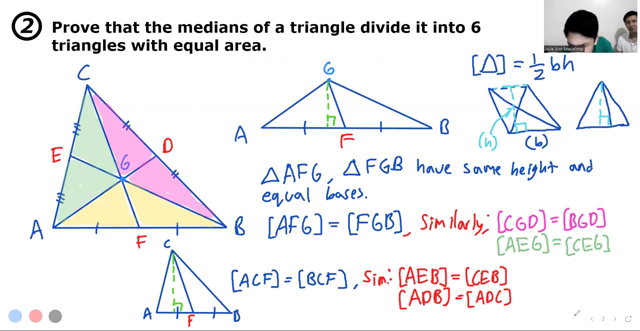 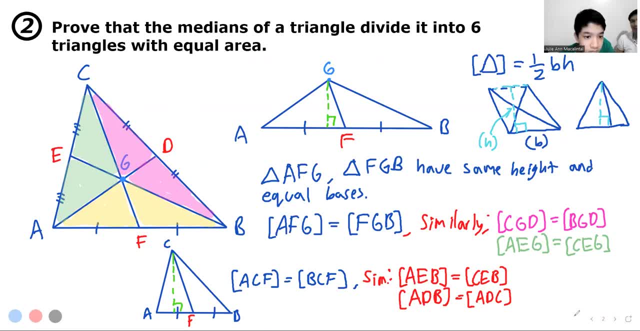 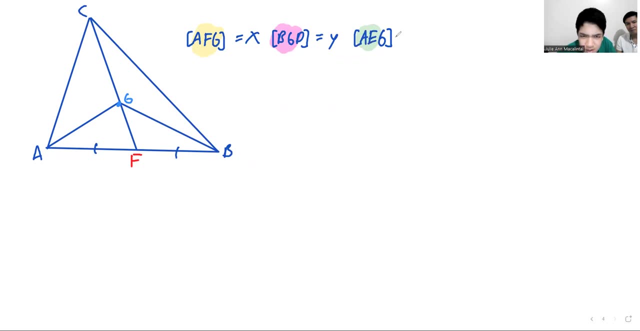 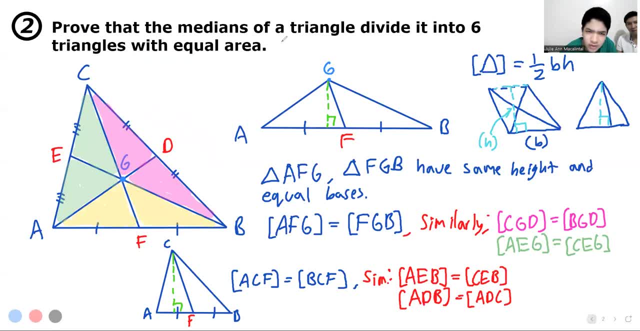 I can, maybe and maybe I should throw at less Let's, let's like that. no, it will be more obvious whom. partially, because maybe you will think that i met the whole area. it's only one small triangle area. they can understand as long as you leave your own triangle. 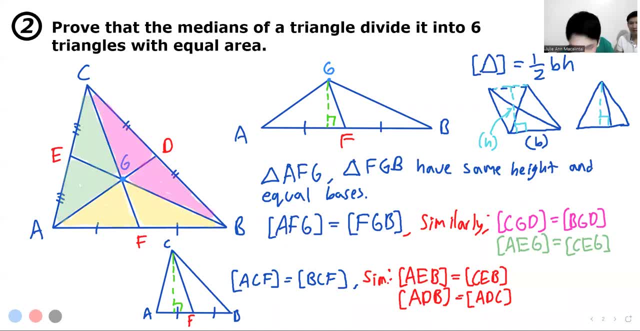 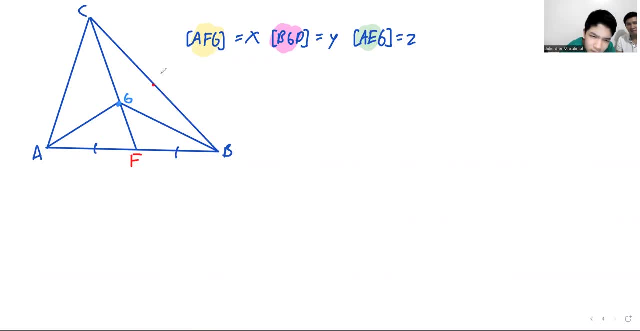 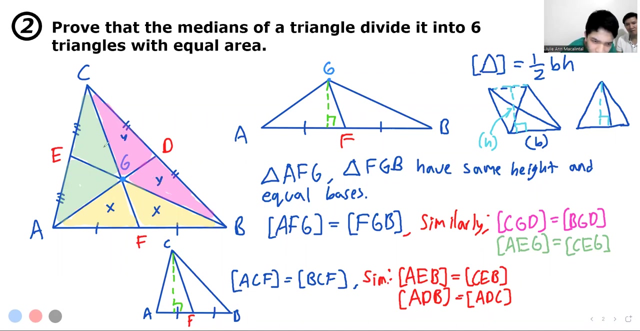 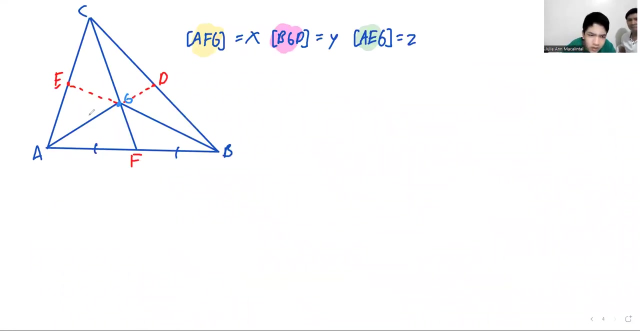 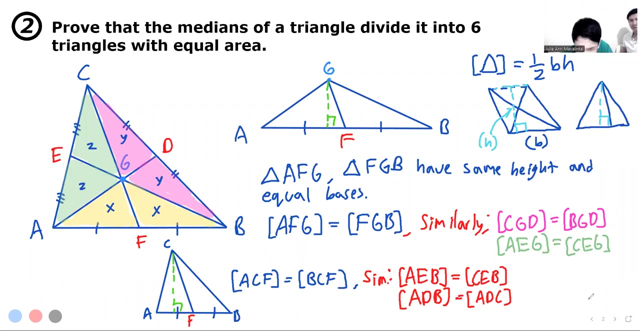 okay, you leave your triangle on the other page because you use these. yes, right, so so this will be x, x, y, okay, so, uh, this will be y and y, v and g, x and y. so earlier i proved that i remember an acf mean tf, yes, so 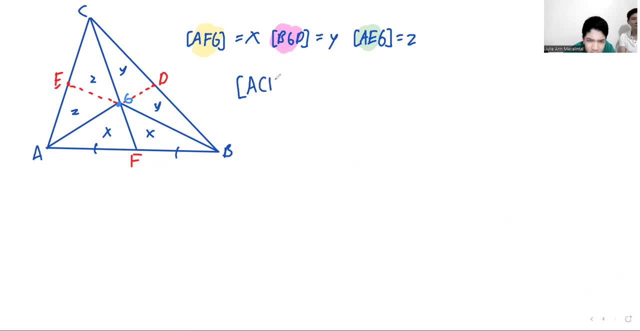 ecf. so this is x. this boozy, it's like wow and oh is equal to x, is to y. Then, therefore, 2z is equal to 2y. Therefore, y is equal to 0.. Okay, so now we just prove this. 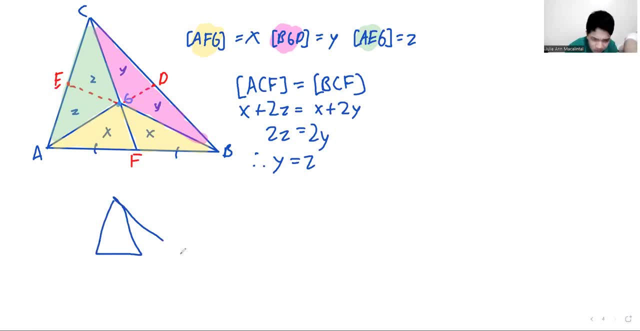 The yellow. Yes, right, I'll just make a quick sketch. This one yellow, Ah, yes, And you got white. No, the purple and the pink, The pink and then the green And the screen green, So one pink triangle. 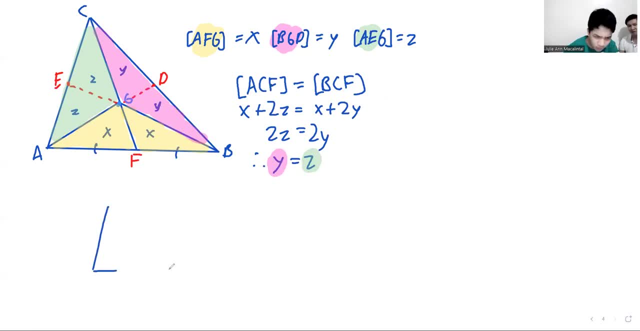 There's an equal area without the red screen triangle. Now what will be the dominating world? the screen green. Similarly, Similarly, Oops, Forgot this word. Similarly, What can we use? We can use any. Yes, Maybe A, E, B, C, E B. 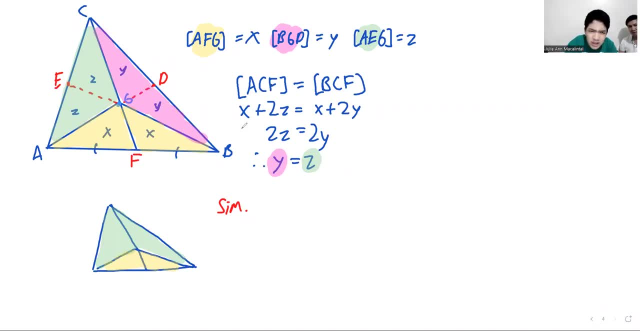 Yes, A E, B, C, E B. When A B, C is the base: Yes, A B, C E, B, C, E B. So this is: What is it? 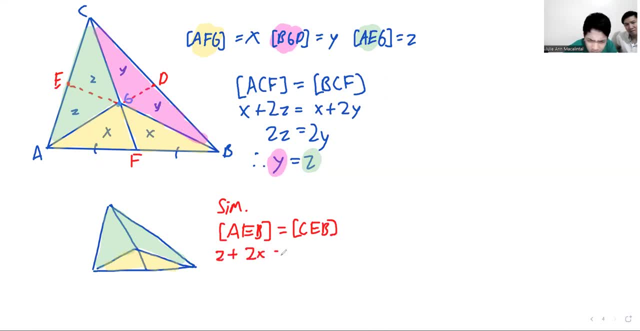 E plus 2X is equal to Z plus 2Y, So therefore 2X is equal to 2Y. Therefore, X is equal to 2Y, So in particular, X is Yes. So now, 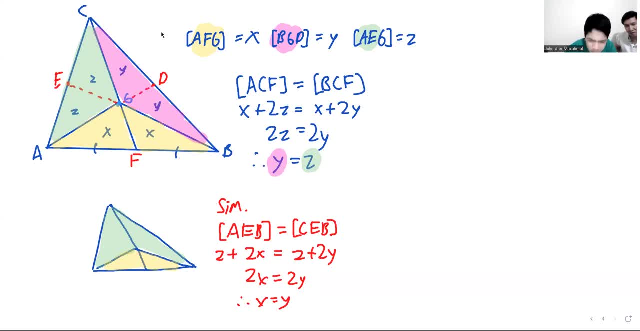 The X And you don't get it? Ah yes, If you want, you can use red X, And this is So. therefore, our entire triangle, One yellow triangle, is equal to area with that of a big triangle. I'm just not doing this. 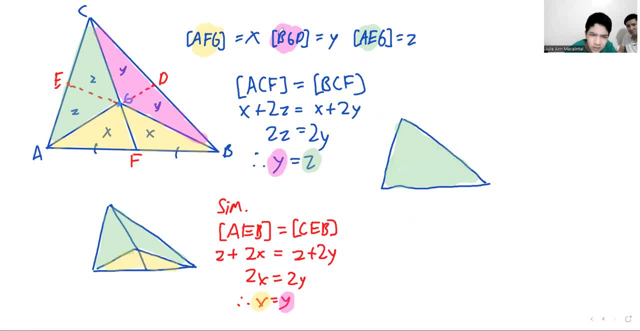 Yes, The entire area is now X, X, X, X, X. this was X X, Z, Z, or it should be. It should be Y. It should be All Y. No, it should be all. 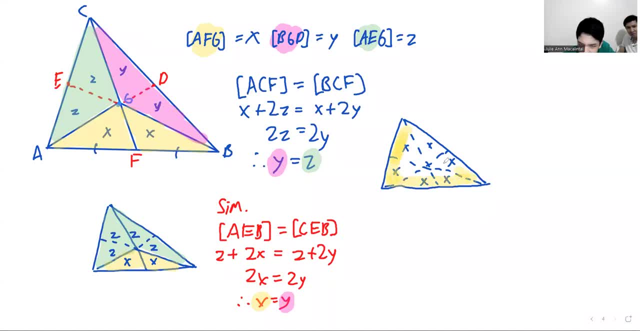 All Y, All Y, Yes, All Y Yes. So I did No, it is equal to both It? Ah, okay, So I will have to use a different No. no, it's the same. 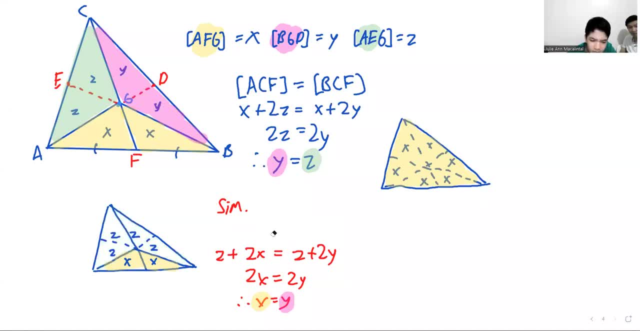 No, This the it's about. Oh, it looks, Thankfully there is control Z, It's Z Okay, All right, So we'll do this. So now, So now, So now. 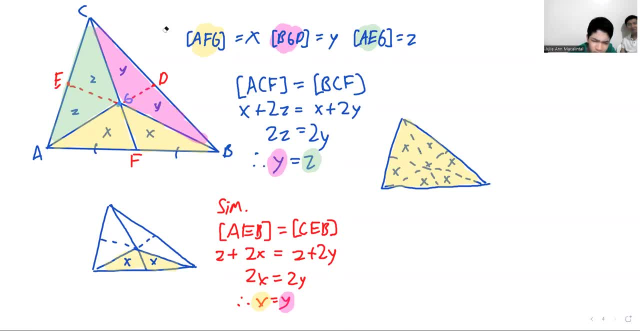 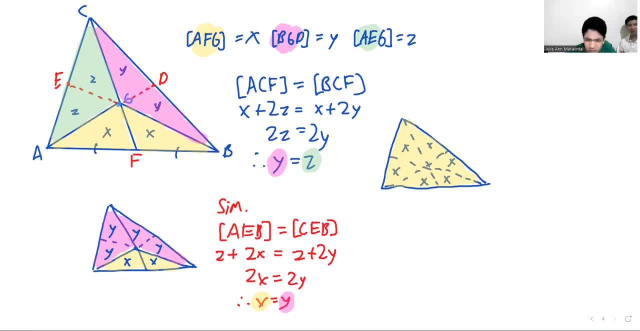 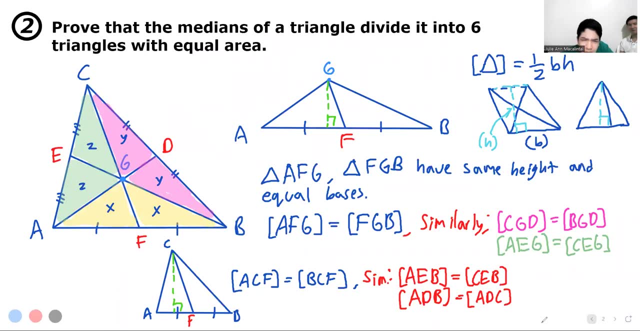 And then now x is equal to y, So they're all x's. They're all x's or they're all y's. Yes, So what is the goal of the problem? The goal of the problem is prove that the mediums of the triangle divided into six triangles with equal area. 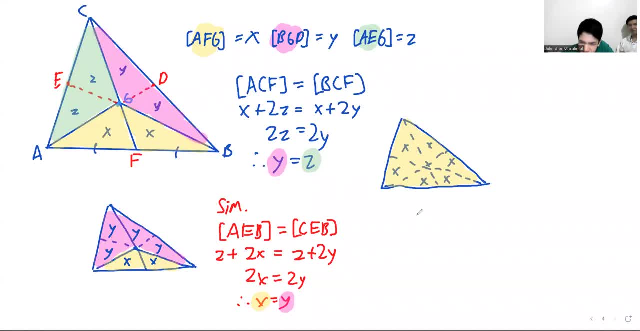 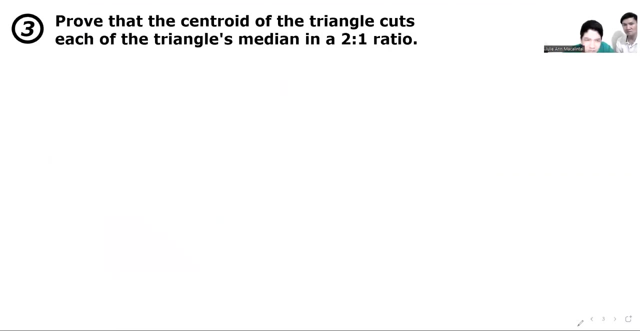 Yes. therefore, This is x, Yes, QA, Yes, Whatever the result. Yes, Nice, Nice. Okay. So our next problem. Can you move quickly? Prove that the centroid of the triangle parts. each of the triangle should be divided into two to one range. 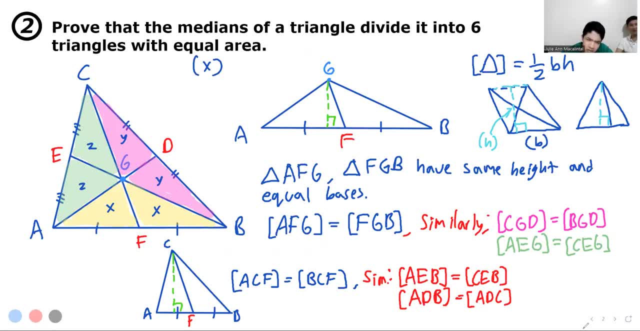 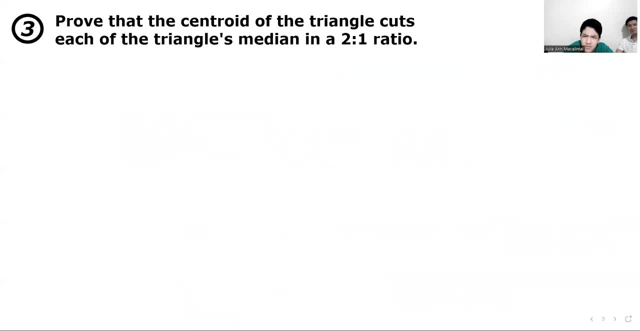 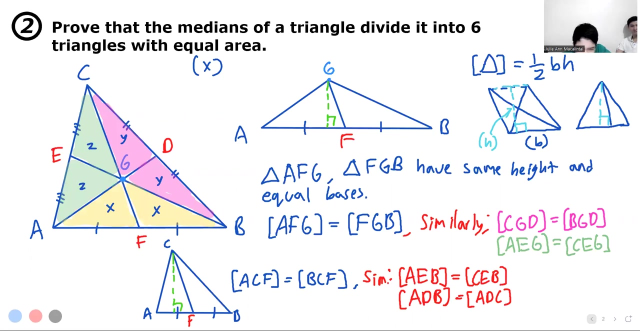 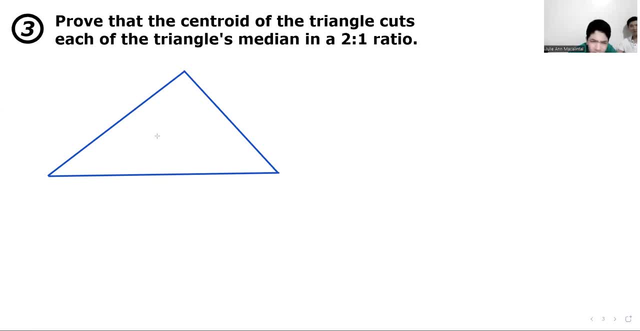 Oops, Okay, Let's see. Here we already proved something. Okay, Where is the demo? Okay, Here we already proved something. Okay, Where is the demo? Okay, Where is the demo Y? Where is the demo? 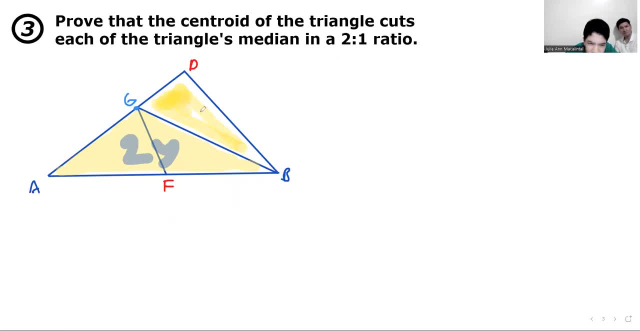 Y, Y. This is, This is If we, If we- Oh wait, no, Should be X, Oh wait, no, Should be X. We can try calculating. The yellow sign is for X. The yellow sign is for X. 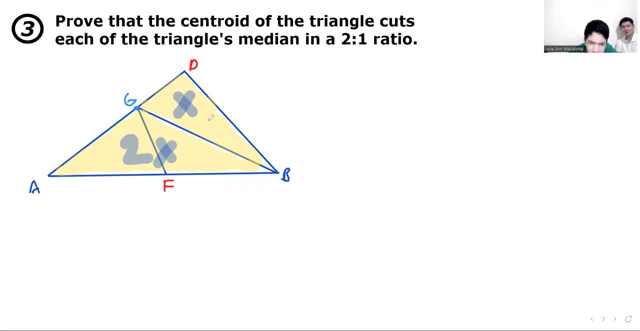 The yellow sign is for X- X. There, We have that is X. We have, that is X There. okay, so now, um, is this all true? yeah, it's a little all clues, so, oops, ah, never mind, doesn't want to exist. 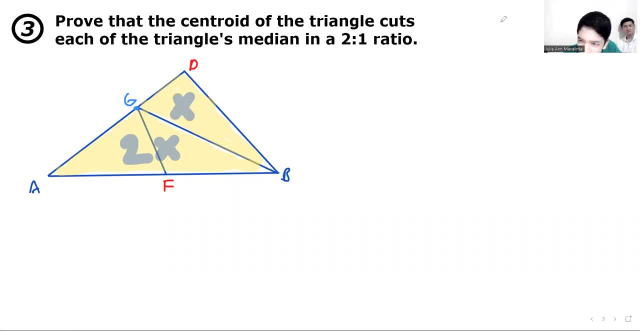 uh, okay, so they have the same height. obviously they cover the same vertex e, so here agb has same height as gbd or dgb there. okay, a, g, b, a, gb. this is a gb is what they don't make me don't know. okay, I'm doing this. 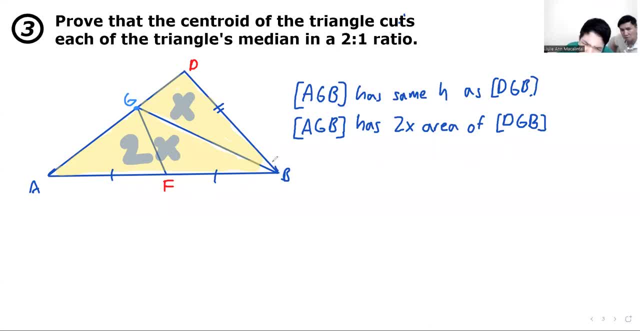 that could be one of these veo. okay, so let me reuse this instead. Yes, so now it will be more apparent. So we're going to prove that this is one and this is two. these are two-times area. So if AGB is one-half B of AGB, this is AGB. I'm going to put it: times 8, equals one-half. 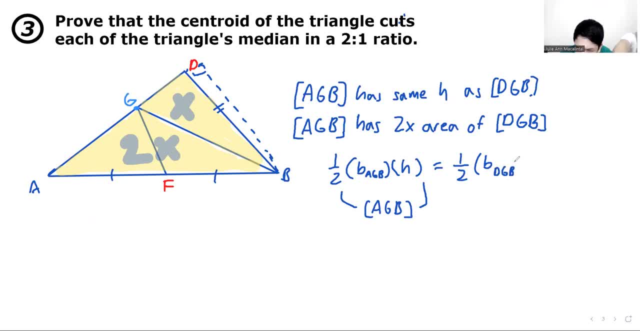 base of AGB. So therefore, AGB is one-half base of AGB. If AGB is still twice DGB, therefore, the base of AGB must be twice the base of DGB. So what's the base of AGB here? 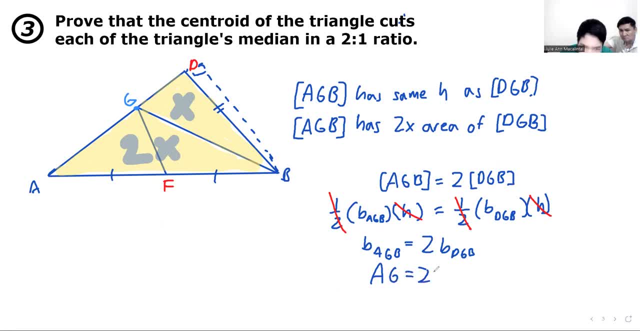 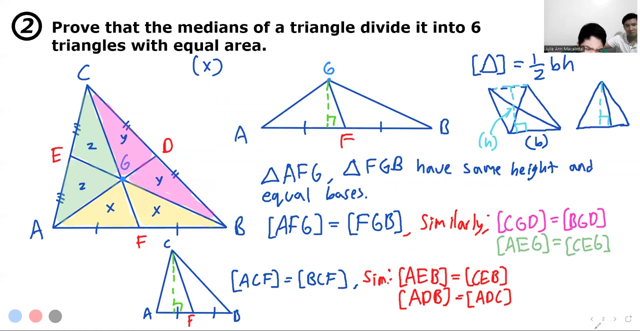 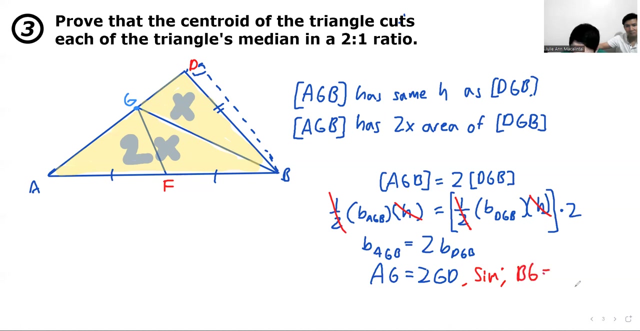 It is AG. AG is equal to two-times GB. Oh wait, Ah yes, Okay, Okay. So AG is equal to two-times GB. Similarly, What are the other medians? BGB, BGB, BGB is equal to two-times GB. 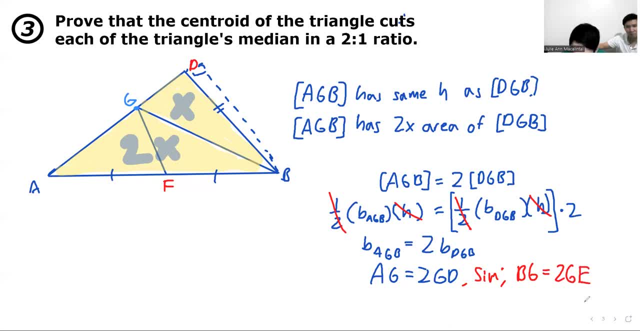 Okay, So you'd say BGB is equal to two-times SOходит electricity. You're right, but what if the number 1 is A and 2 is U? so what would that be? Yes, B, GB, B 19 would be 0..